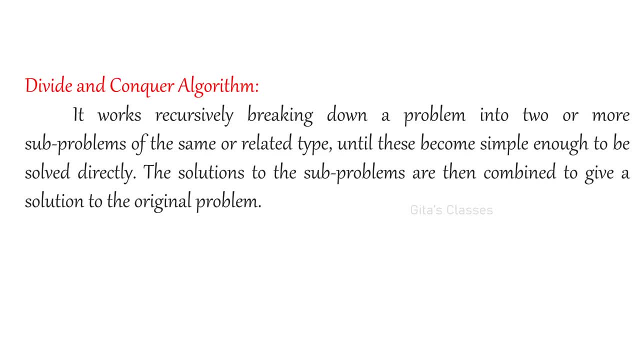 big. if you are not able to solve, then you can divide them into sub problems of the same type or related type. okay, then it will become very simple. till we get it simple, you have to divide them. then the solutions of the sub problems we can solve the sub problems each sub problems can be. 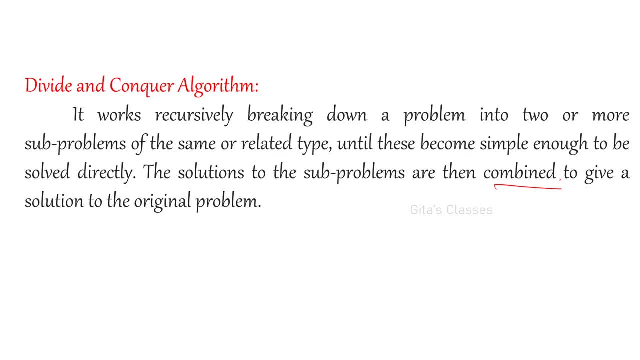 solved separately, then they have to be combined from the name itself. you can understand divide and conquer. if the problem is very big, then recursively you have to break down the problem into two or more sub problems of the same or related type. okay and very simple. it is very easy. let us see. 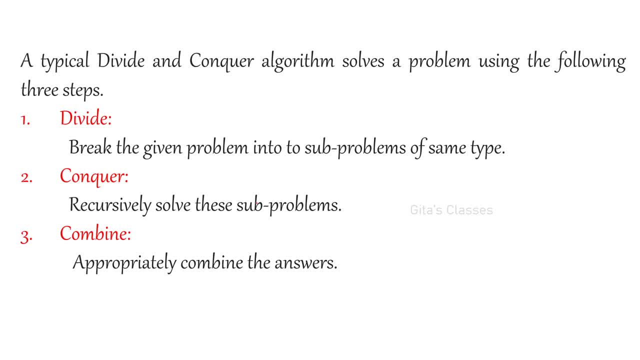 a typical divide and conquer algorithm solves a problem using the following three steps. three steps, sorry. so first step is divide, break the given problem into sub problems of same type, then conquer, that is, recursively solve the sub problems. okay, so our problems are solved, the sub problems are solved. 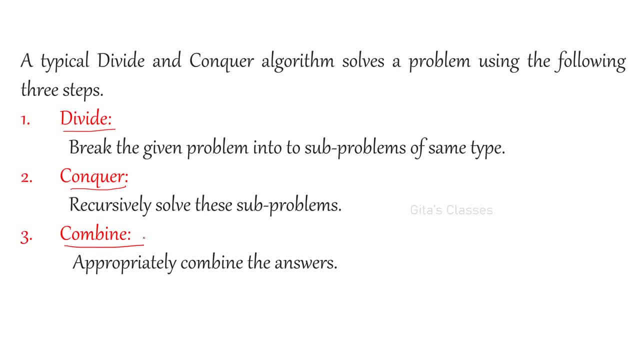 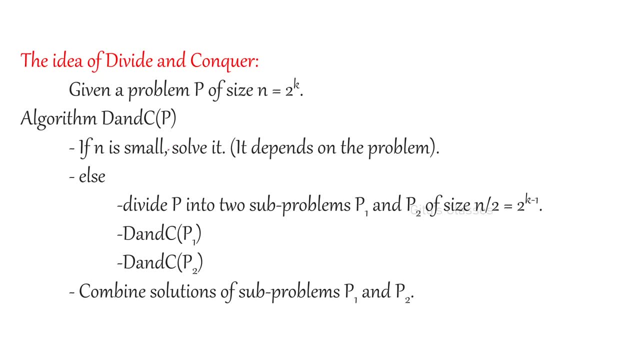 again appropriately combine the answers. okay. so now the idea of divide and conquer. if you want to write it as an algorithm, then assume that given problem p of p is of size n. for our convenience, let us take it as 2 power, k. okay, and the algorithm d and c. according to the textbook, it is d and c. 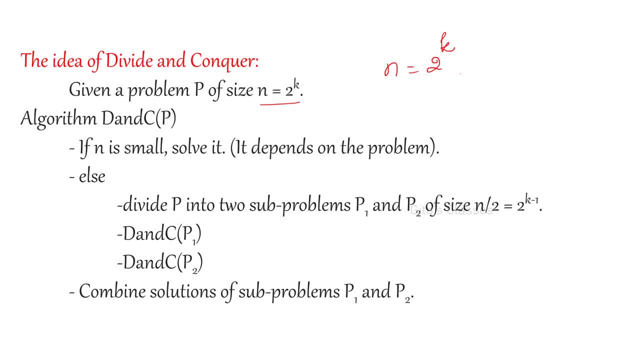 of p. it is calling the problem p. okay. so if n is small, solve it. it depends on the problem. what you mean by this? small depending, exactly, depending only on the problem. for some problem n is equal to 1. may be small. for some problem n is equal to 5. 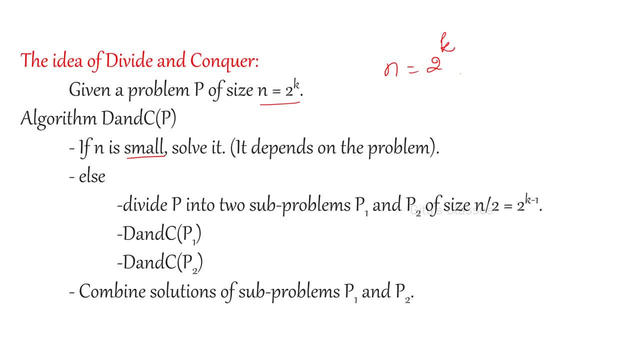 may be small. for some problem, n is equal to even 20, maybe small, okay. so, depending on the given question, it if it is. if you feel that it is small, then solve it directly, okay, otherwise, else else, what happens? divide if it is not small, if it is, if. 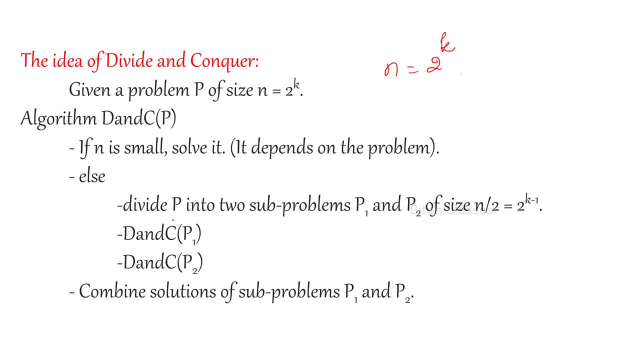 are not able to solve it directly, then divide p into two sub problems, p1 and p2. of size n by 2. n by 2 means here you have 2 power k. we have assumed that n is equal to 2 power k. therefore n by 2 means 2 power k minus 1. okay, now you solve these two. generally it is of size. 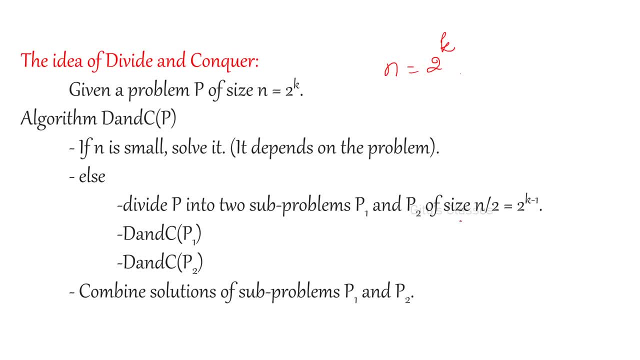 equal size, but sometimes it may not be of same size also, sometimes it may be different also. so now you have to solve p1 using this algorithm. that is, again it is calling the algorithm: okay, divide the sorry, solve the p1. okay, then similarly solve the p2 sub problem p1 and. 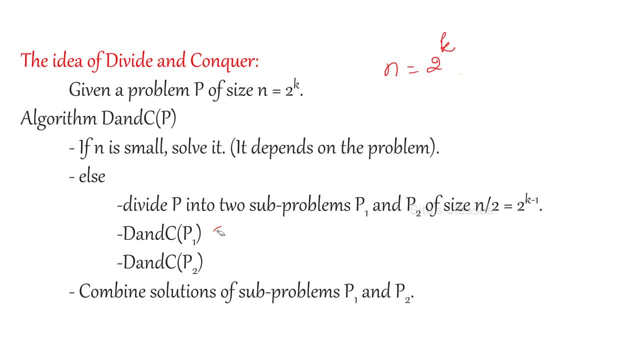 sub problem p2 are solved using the same algorithm. okay, then again, after solve, now we got the solutions of these sub problems, solutions of p1 and p2. we got. okay, using the same algorithm. using the same algorithm, got we have solved p1 and p2. now you have to combine. we want the solution of p only, right. 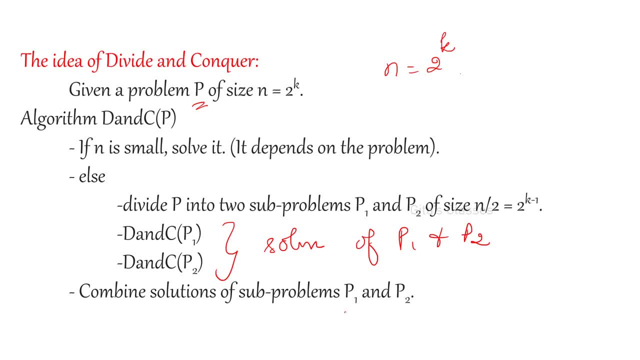 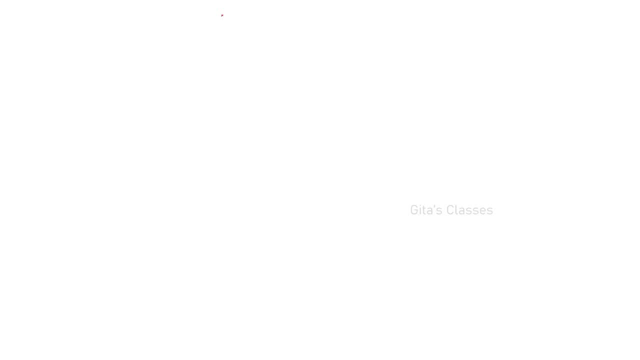 so combine the sub problems, combine the solutions of sub problems p1 and p2. okay, now let us see actually what is what you mean by here. again i will explain here. p is the given problem of size. n is equal to 2 power k. for our convenience let us take it as 2 power k. so if p is very small, 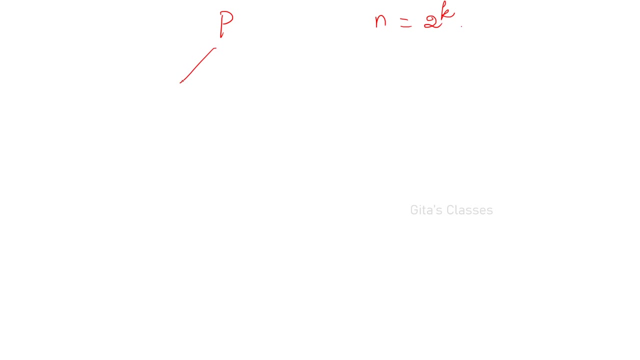 if you can solve it directly, solve it. otherwise you have to divide into two sub problems, p1 and p2 of size. what will be the size? it is 2 power k minus 1. okay, equal size. assume that we are solving it, dividing it into two equal parts. so, again, p and p1 and p2 are small. then solve them. 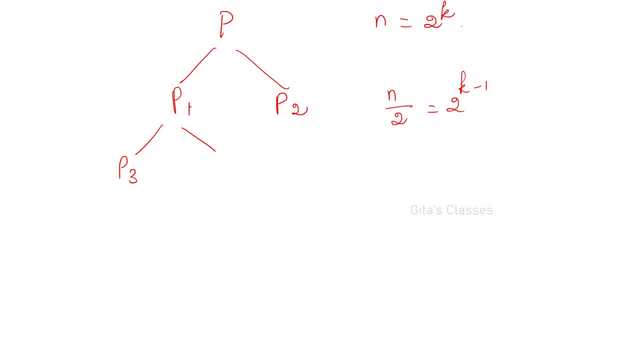 using the same algorithm. you can solve them. otherwise, if p1 is large, it is not heavy. if you are not able to solve that, again, divide that into p3 and p4 and p2. also, if you cannot solve you, divide it into p5 and p6.. What will be the size of these things? Again, n by 4, right? so? 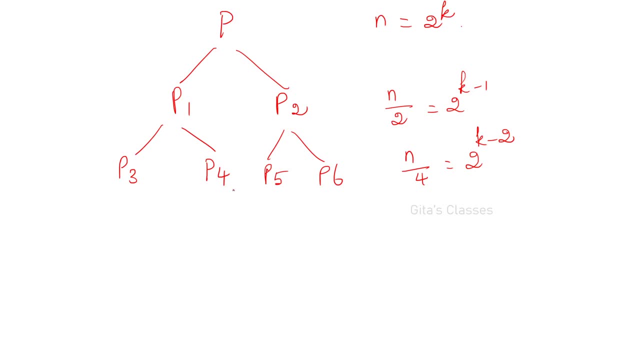 2 pi k minus 2.. Then again, if p3, p4, p5, p6 are small, then you can solve. otherwise you have to again subdivide into sub problems of p3, that is, p7 and p8. each one can be divided like this: 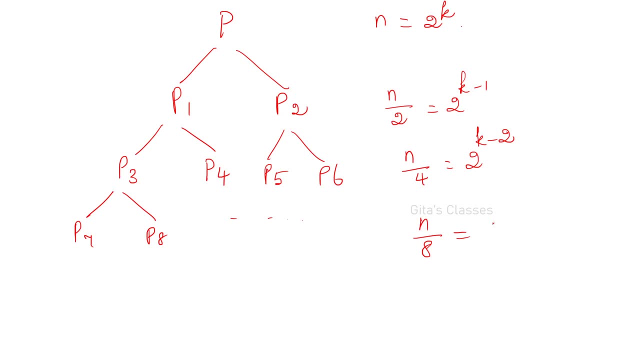 What will be the size of this one? n by 8, right, that is 2 pi k minus 3, and so on. till which step you will be able to divide, till you get all the values are 1 1 1, 1. okay, So this is what is the. 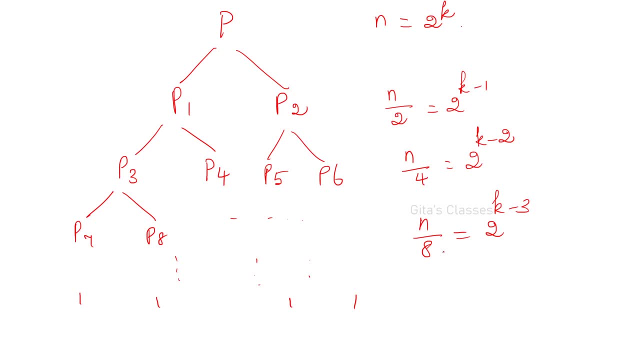 height of this is a typical tree, Right? so what is the height of the tree you will get here, till which step you can go? k. so the height of the tree will be is k? okay, k levels you will have. this is level 1, level 2, level 3. so how many? 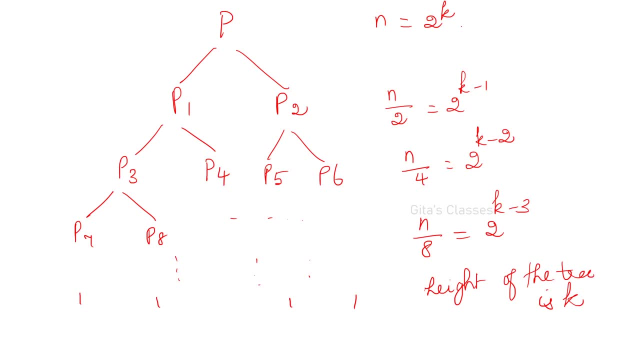 levels, you will have. k levels, you will have. okay, so height of the tree is called k. Now, divide and conquer is typically implemented recursively here. Okay, one after the other recursively, which results in a tree of recursive calls. Actually, for solving p1, we will call p. only, the call algorithm is p. okay, the method of solving. So if this is small, 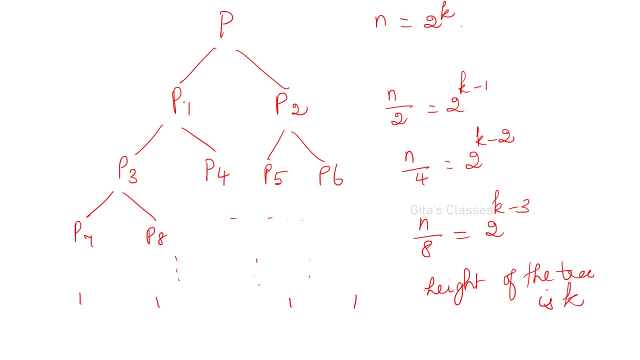 you solve it otherwise, divide them into two and this- p1 and p2- can be solved using the same algorithm, same method. okay. Similarly p3 and p4. all these they are calling recursive. it is a tree of recursively, as we have seen in this example. okay, So now how long it will take, actually, how? 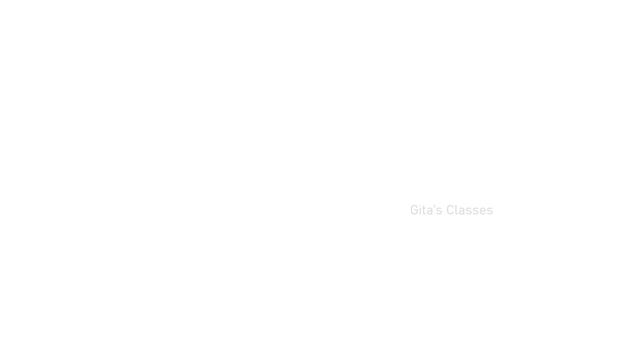 long this divide and conquer time? how much time will it take? how many times now we are going to see? how many times do we need? do any elementary operations okay? or such as comparison or any other operation? it depends on the algorithm, okay, So let us assume the given problem is t of n. 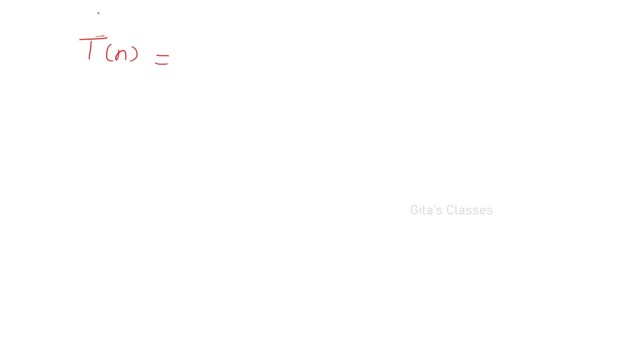 If the given problem is t of n, now you are dividing this is for p. okay, now you are dividing it into two equal sub problems, that is, of size t of n by 2 plus t of n by 2. right Now, after solving, what will you do? actually, how much time it will take, time for solving the problem. p is equal now time. 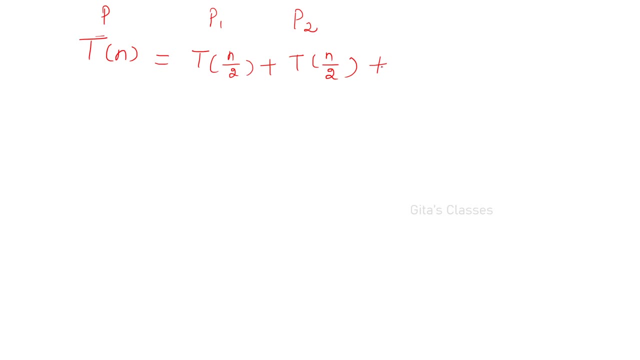 for solving p1 and time for solving p2 and you will get an additional time. that is additional cost for combining these two solutions. Now, p we have divided into two sub problems. if you solve p1 and p2 again we have to combine the solution no. So this is called. 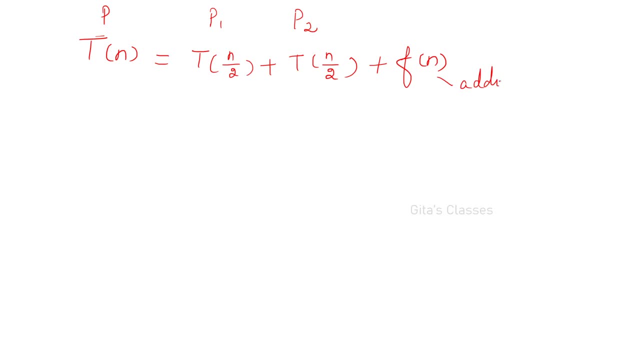 additional cost for combining. okay, So, fn. so this is additional cost of combining, and here we are assuming that for dividing there is no extra cost. okay, It is a constant. we are assuming in that it is a constant. So now we can write it, as t of n is equal to 2, into t of n by 2. 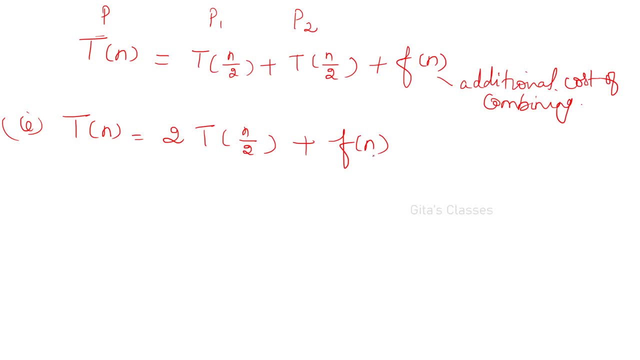 plus f of n. okay, So here this example: we have divided the problem p into two equal sub problems. okay, Sometimes it need not be equal, sometimes it may be different. okay, So in general we can write it as t of n is equal to 2 into t of n by 2 plus f of n. okay, So here this example we have. 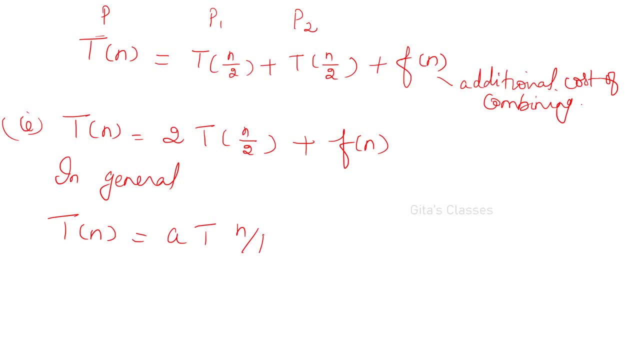 equal to a into t of n by b, n by b plus f of n. Here, if you divide it into two equal parts, then n by 2. here it is not like that it may be divided into three parts, four parts, etc. okay, and for combination a: okay, and these need. 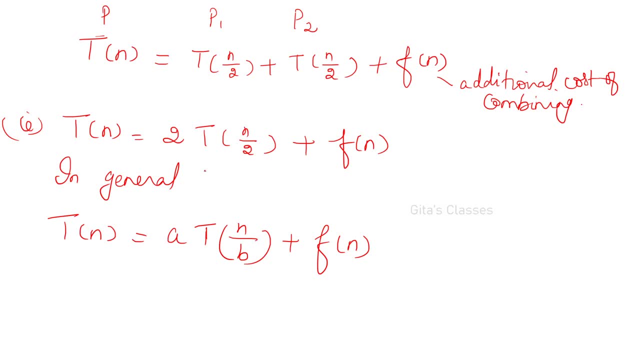 not be equal always. okay. Sometimes if you divide, one may be able to solve. you may be able to solve one part. the other parts can be ignored. something like that you will get okay. So this is the typical recurrence relation. t of n is equal to a into t of n by b plus f of n is the recurrence. 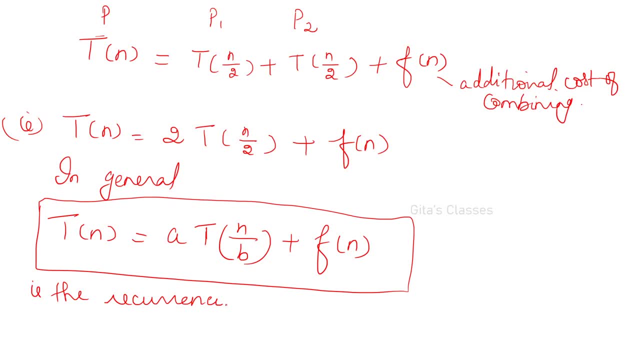 relation. This is an important part of divide and conquer algorithm: recurrence relation for a divide and conquer algorithm. Okay, So now let us solve this equation. Let this be equation number one. This is recurrence relation for divide and conquer algorithm. So solving this for: a is equal to 2, b is equal to. 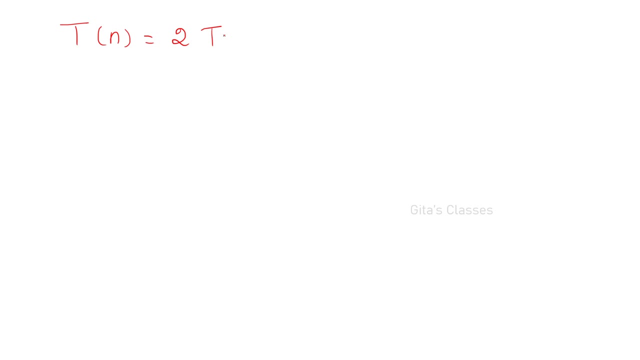 2. Now we have seen t of n is equal to 2 into t of n by 2 plus n. Now this is n is linear. Okay, This is the cost of combining this f of n. Let us take f of n as n. Okay, Now let us solve. 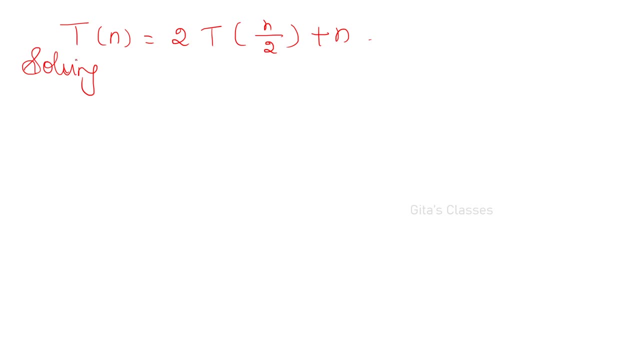 this using iteration method. Solving this recurrence relation using iteration method or substitution method. you can say: Already, we have seen how to solve this recurrence relation using iteration or substitution method. How will you solve? You keep on substituting, right, So t of n is equal to 2. into see what is t of n. 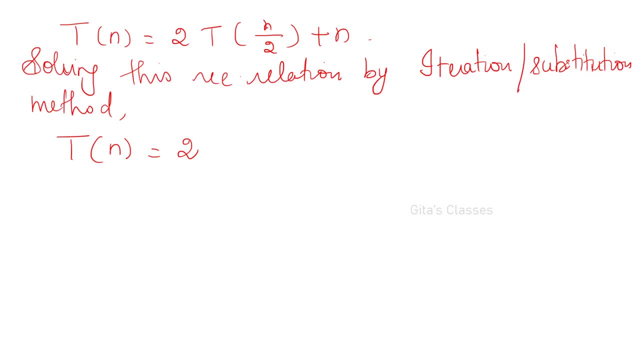 twice t of n by 2. You divide it by 2.. So in the place of t of n by 2 twice, you divide this by 2. So t of n by 2 into 2, that is, n by 4.. 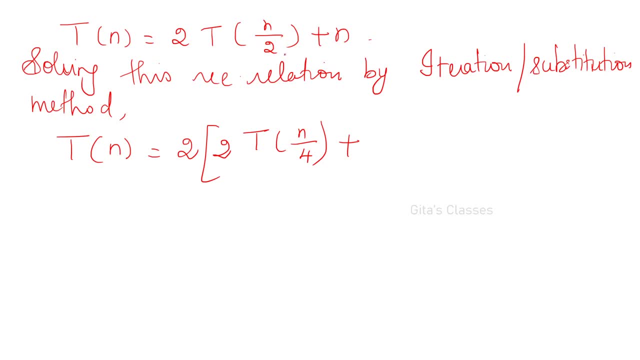 Plus here. if you have n here, you have n here. Now we have n by 2 here, So I will write n by 2 here. Okay, Plus n. So if you expand it, this is 2 square, that is 4 into t of n by 4 plus 2 into n by 2. you. 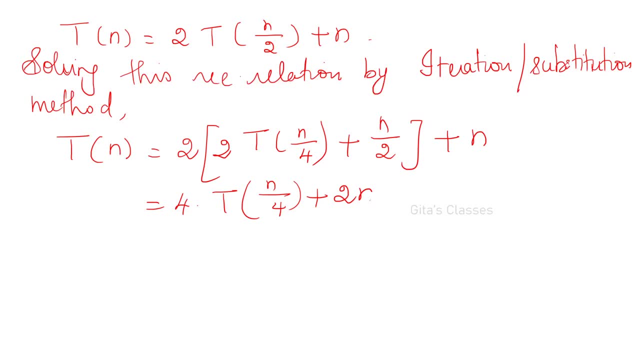 will get 1 n and here one more n. Therefore it will become 2 n, Right? Similarly, what will be the next one? Again 8 into t of n, by Again twice t of n by 2 into 4.. Okay, So t of n by 8 plus 3 n. You observe like this in general. I can write it as: 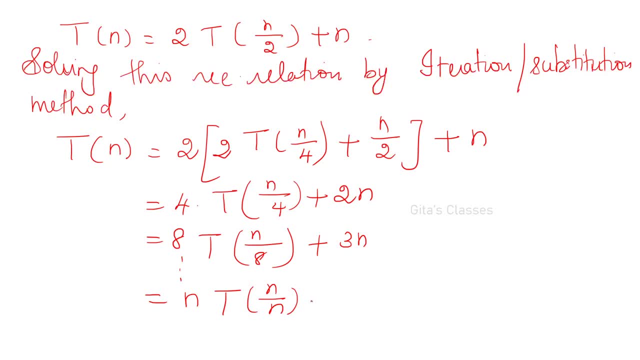 t n into t of n by n, plus how many times. see remember: 2 power 1,, 2 power 2, 2 power 3, etc. n is equal to 2 power k. We have assumed that n is equal for our convenience. I told you n is equal. 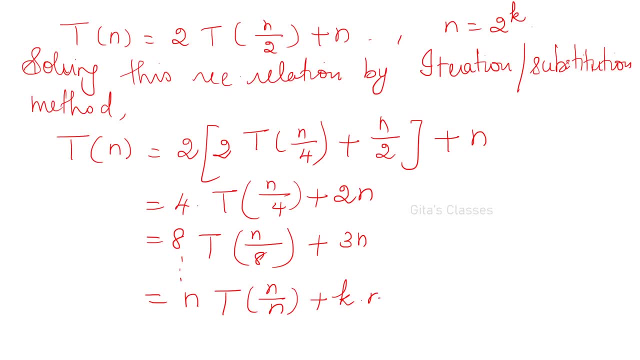 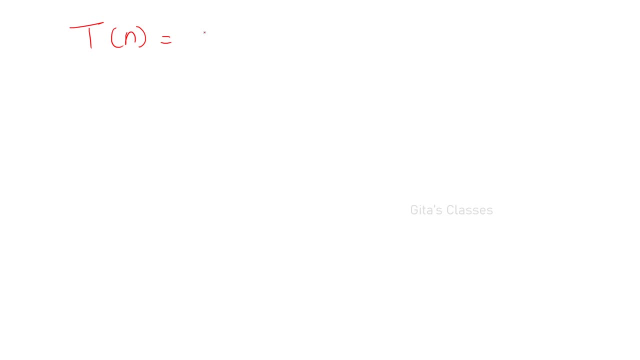 to 2 power k. So what will be the value you will be getting here k into Right. Therefore, t of n is equal to n into t of 1 n by n, that is 1 plus k, into n, k times n. 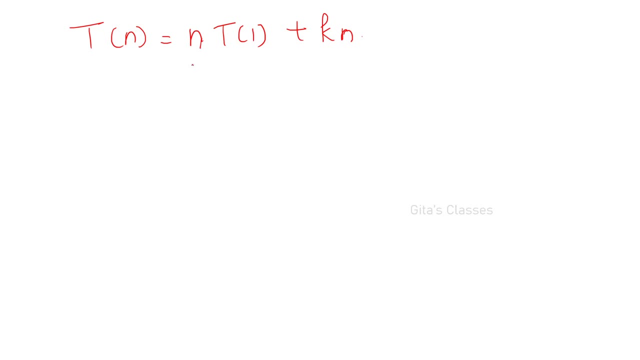 Okay, So first is n times t of 1 is a constant. So this is a constant. This is a constant time n and this is k into n. What is our k times n? This is k times n. Actually, n is equal to 2 power k Right Given. n is equal to 2 power k Implies. k is equal to. 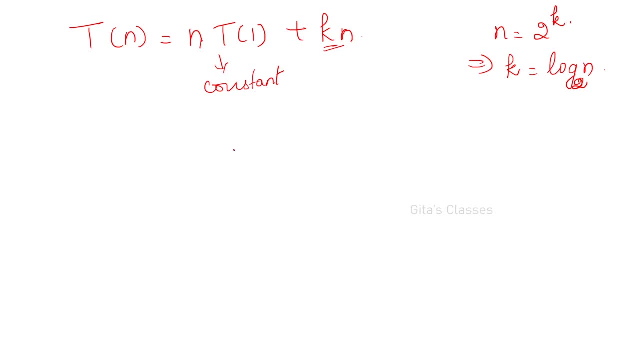 log n base 2.. Okay, K is equal to log n base 2.. Therefore now, comparatively, this first term is very small, So we can ignore that. Okay, First term can be ignored because it is very small compared to the second term. Therefore we can write it as: t of n is equal to n into. 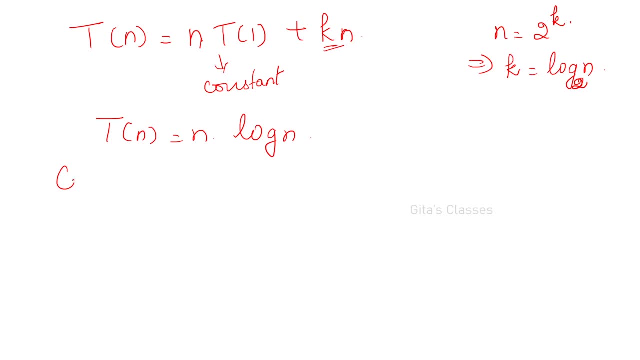 log n. Okay, So the complexity is: is O of n log n? Okay, So for divide and conquer algorithm, if n is linear, then we can write it as n log n. It is understood that here in computers generally log n means log n base 2.. Okay, It is base 2. that is why, if you want, you can write n log n base 2. 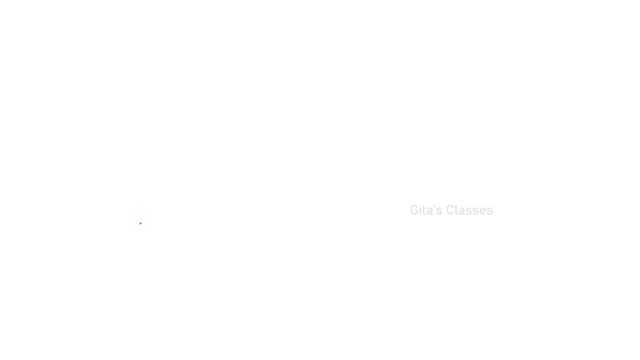 also Now. So in general we have seen t of n is equal to a into t of n by b. This is the general recurrence relation, Right? So when this is the general recurrence relation, we have taken it as 1.. So when a is equal to 2, b is equal to 2 and f of n is equal to n, which is linear. Just now we 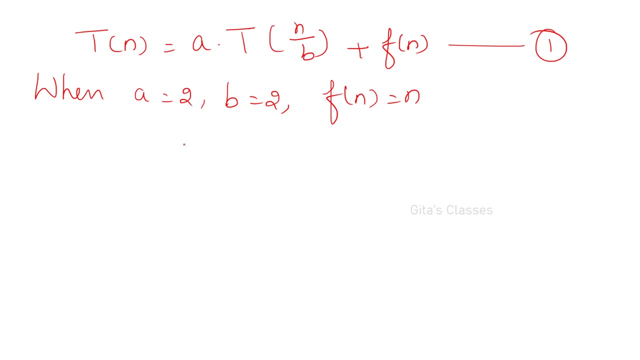 have solved this Right. What is the complexity? we got O of n log n Right. This is one example. Let us see one more example, Example 2.. When n is equal, when a is equal to 1, b is equal to 2 and the f of n is equal to constant. That is the combining. 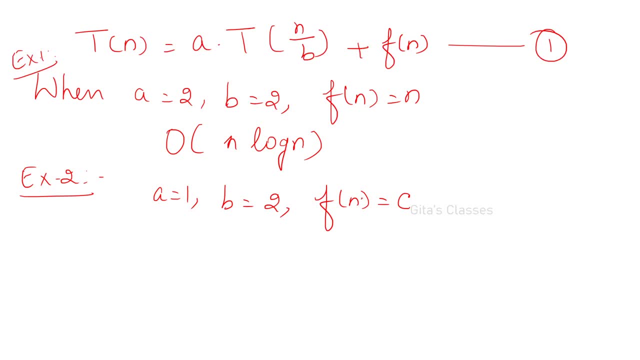 combining the solutions will be constant. Okay, So divide it into two sub problems. Okay, b is equal to 2 means two sub problems and solve the other. Actually, here one will be. one can be ignored. So a is equal to 1.. That means only one part we are going to solve. The other part can be. 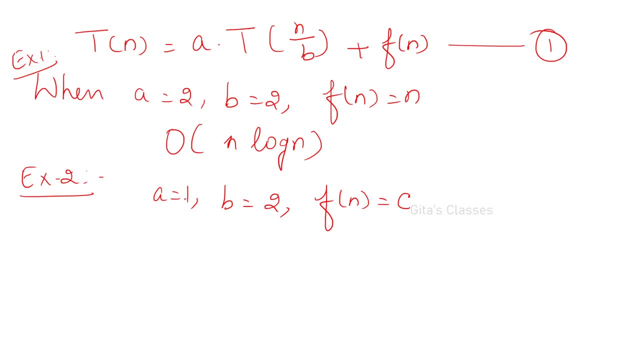 ignored. Okay, So in this case, a is equal to 1, b is equal to. There is no need to combine the solutions, Only one solution. That is why we have taken f of n is equal to c. Okay, So t of n is. 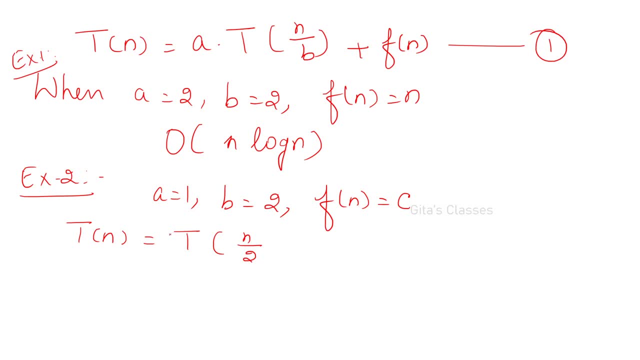 equal to 2.. Okay, So t of n is equal to 2.. Okay, So t of n is equal to 2.. Okay, So t of n is equal to t of n by 2.. 1 into t of n by 2 plus c. Okay, So t of n is t of n by 2 plus c. So again, if you divide, 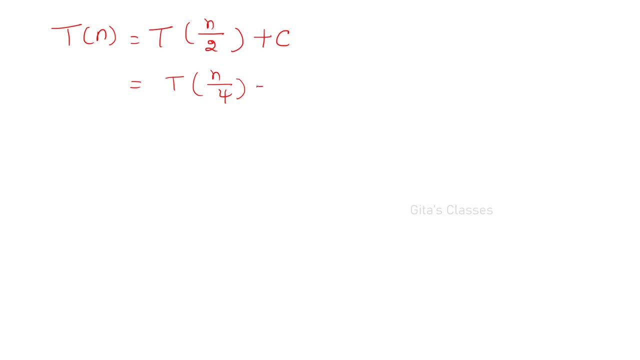 this t of n by 2 means t of n by 4 plus c. For t of n by 2 plus c, Again one more c we have here. That is t of again. t of n by 4 can be written as n by 8 plus c. Again we have two c's here. So 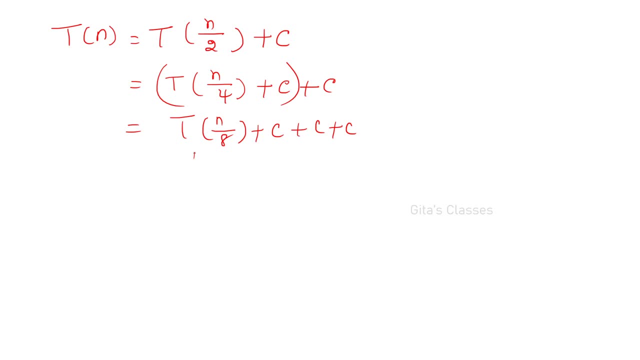 c plus c plus c. So in general, t of n by n plus how many times you will get c k times. See here: 2, 2 squared, 2 c, 3, 2 cube, 3 c and so on. Okay, So this is equal to t of 1 plus k times. 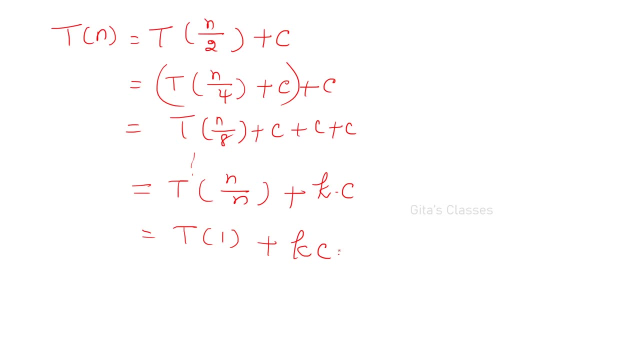 c. Okay, So t of n is equal to, and here t of 1 can be ignored, So n is equal to 2 per k. we have taken So always: k is equal to log n. So here log n into constant time. Therefore. 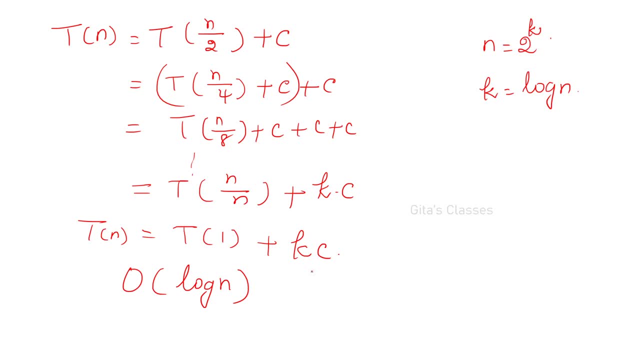 the complexity will become: O of log n. is the complexity Okay? O of log n? we got This second case. I will give you one more question and you can try doing this. So in an algorithm, in an algorithm, we divide large problems. in an algorithm, we divide large problems into three equal parts. 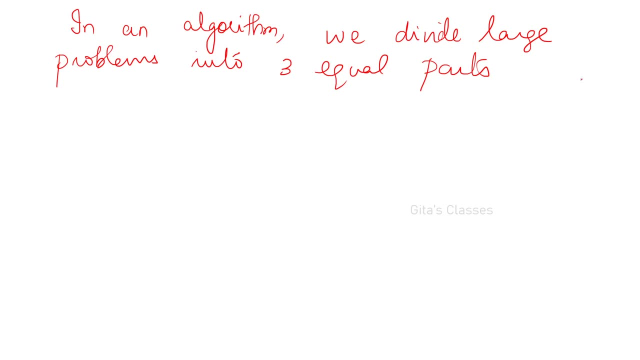 three equal parts and divide large problems into three equal parts of questions. What is the complexity of this algorithm? for size n, For our convenience, let us take it as 3 power k, because we are dividing it into 3 equal parts. Let us take 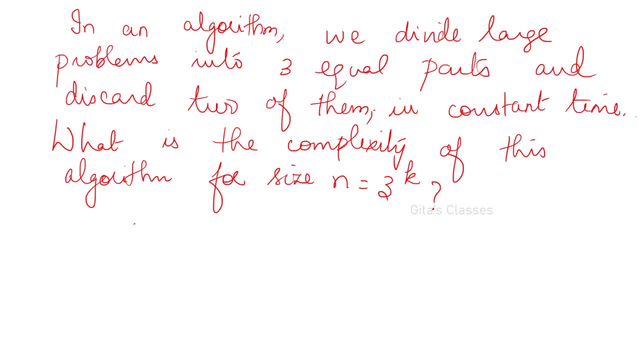 3 power k. So how will you solve this? Here t of n is what 1 into a is 1. here b is 3.. 3 equal parts, and 2. See n is divided into 3.. So given b is equal to 3 and we are solving. 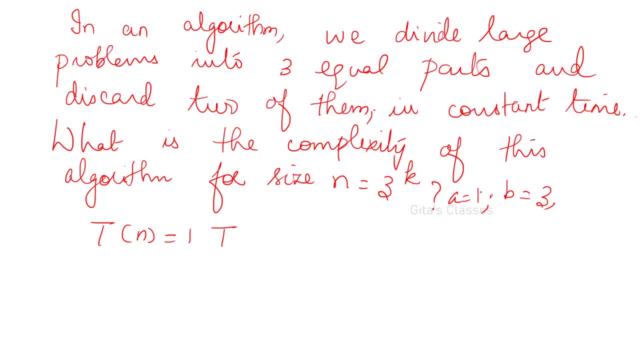 only one part, So a is equal to 1.. a is equal to 1, b is equal to 3.. And how much time it is taking c. So f of n is equal to c In constant time we are solving, So t of n is. 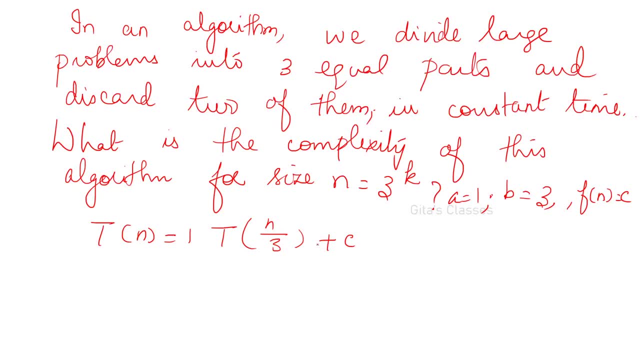 equal to 1 into t of n by 3 plus c. So this can be written as t of n by 9 plus 2 into c. In general we can write it as a t of n by n plus k times c, That is t of 1 plus k. 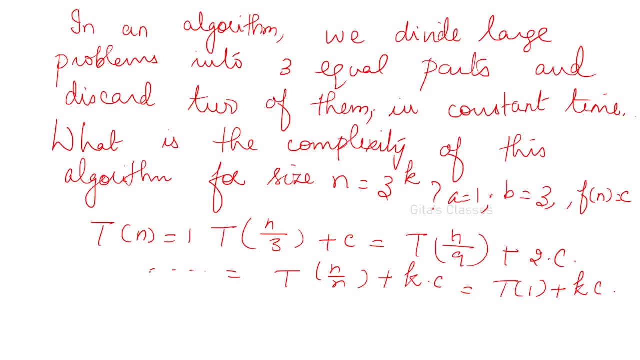 into c. Can you tell me what is k now? Log n base 3 right, Where k is equal to 1 into k is equal to log n base 3, because we have taken n is equal to 3 power k, Right. Therefore? 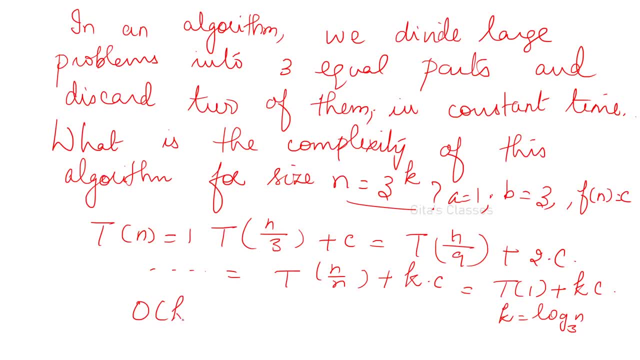 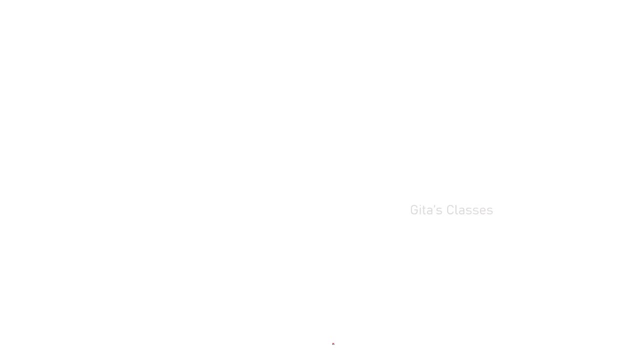 what is the complexity now? Order of k, O of k, Ok, O of k, Or you can say O of log n base 3.. Ok, So now let us see one example, Actually examples of This. divide and conquer algorithms can be used, or some searching We can use it in. 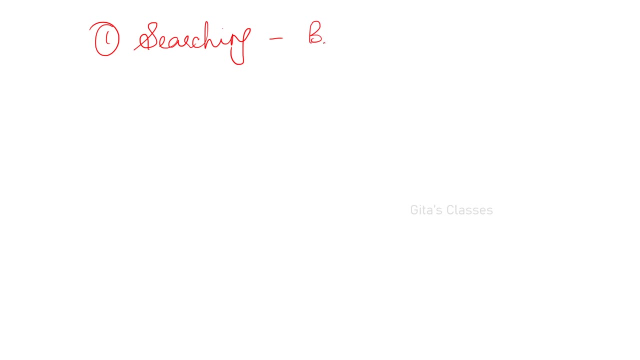 These are all the examples for divide and conquer algorithm. You can say binary search in searching Binary search And second one you can use it for sorting. In sorting we have merge, sort And quick sort. All these algorithms you would have studied already. And tree traversal In tree traversal. 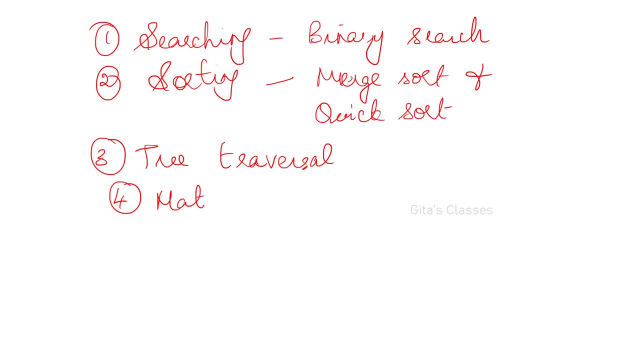 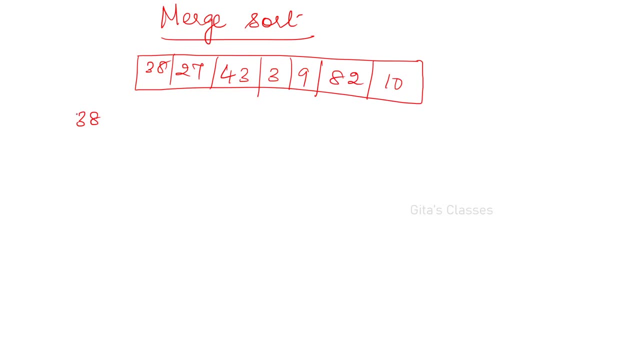 14., 1., 0., 4., 6., 6., 7., 15., 10., 31., 12., 4., 16., 14., 16., 22. 15.. 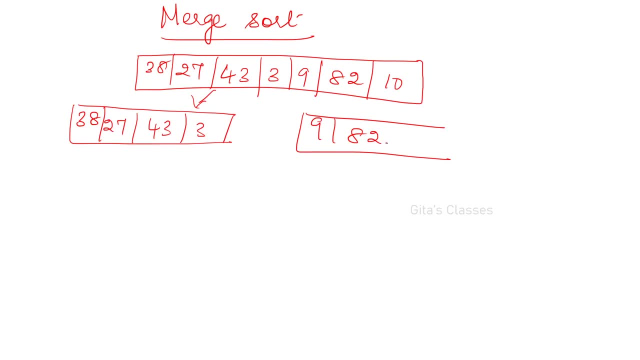 0. 13. I will take 9,, 82 and 10. Right In the second part. Now again I cannot solve. You divide it into again two equal parts, That is 38 and 27.. Then 43 and 3.. 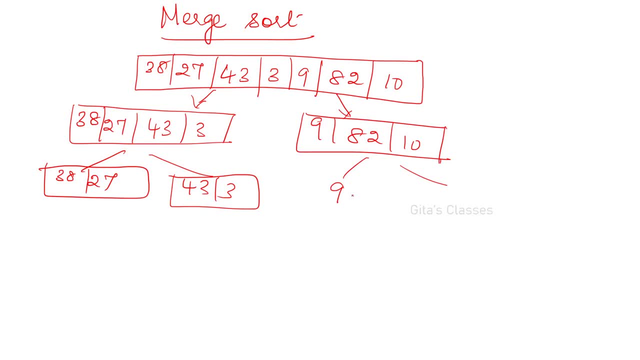 Till you get one element, So 9 and 82., Then 10. Then again divide it into 2. That is 38., Then 27., Then 43 and 3. Then 9 and 82., Then 10.. 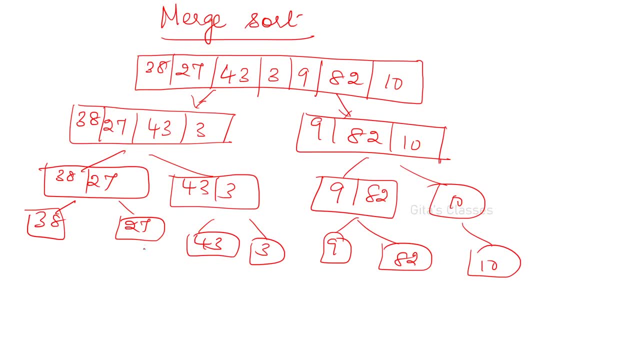 Now we have divided into equal, That is, up to 1.. Now what you have to do is You have to combine these two by solving. What is the solution here? You have to arrange them in the order, So 27 and 32.. 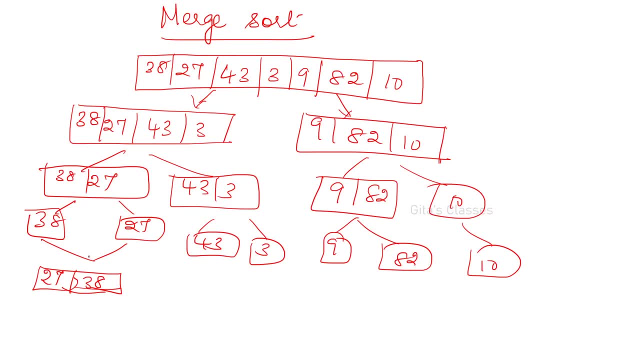 Then 48. Arrange them and combine. Okay, Then here 3 and 43. You arrange them in the, You sort them and then combine Here 9, 82. Then 10. only These two are combined. Next you have to combine 27.. 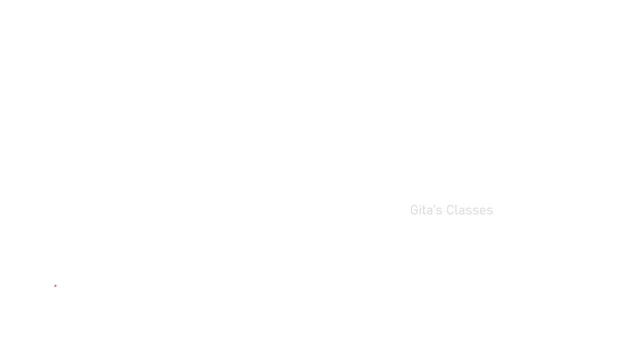 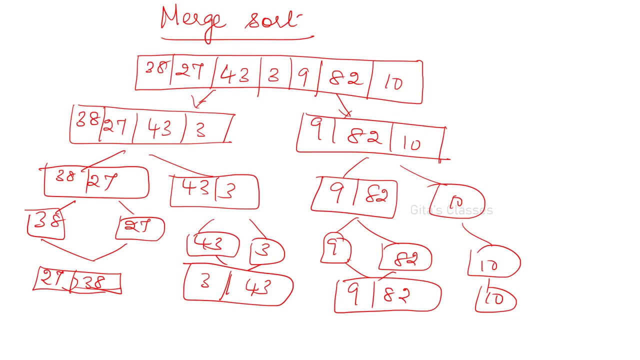 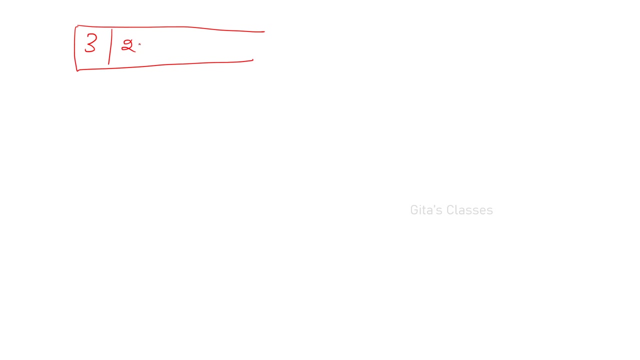 You have to combine these four, Right, Right. So after Combining these four, You have to start these four numbers, Then combine Okay, So you will be getting 3.. 27. Then 38. And 43.. 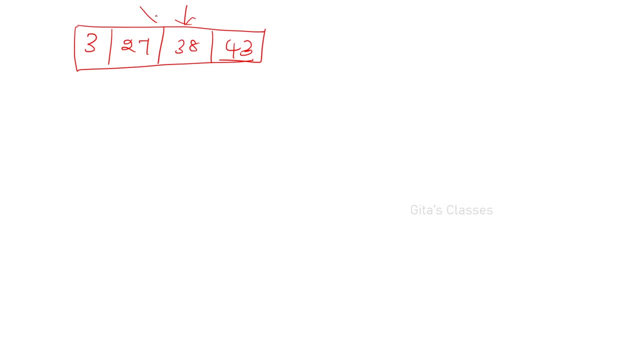 Right, This is from the previous one. Combination of these two, Okay, The previous two. Then again here in the next part, 9, 10 and 82. Then you have to combine. Combining these two, Ok, Combining the from the previous two. 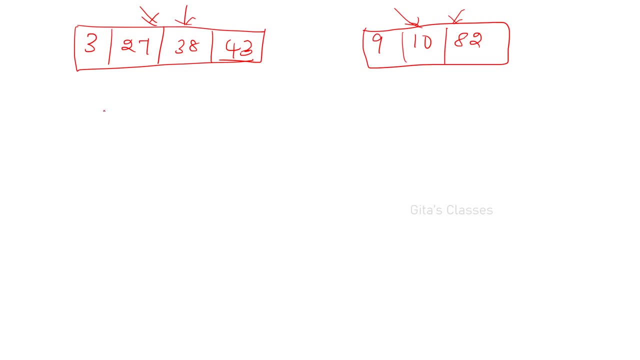 Now again, you have to combine these two By arranging. That is, you solve them, Then arrange, So 3. You will be getting 3.. 9. Then 10. 27. 38., 43. Then 82.. 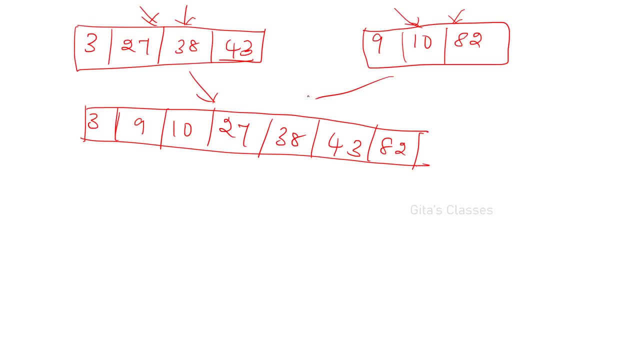 okay, so this is a typical example of divide and conquer algorithm. okay, this is much sort so like this: for everything, you have to divide them into sub problems, then you can solve them, then combine. okay, and we have seen the recurrence relation for this divide and conquer algorithm. 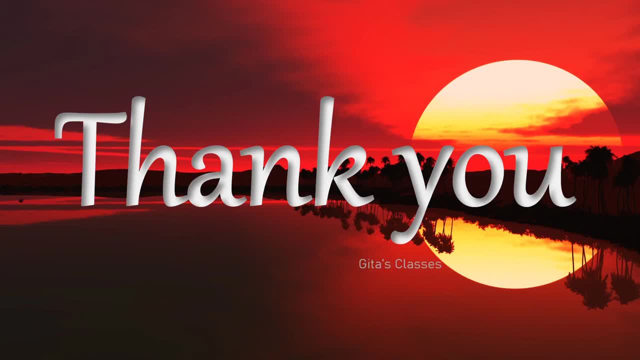 also, you can solve the recurrence relation also with this. unit 4 is over. next we will start graph theory in the next class. that is unit 5. okay, thank you so much for listening.